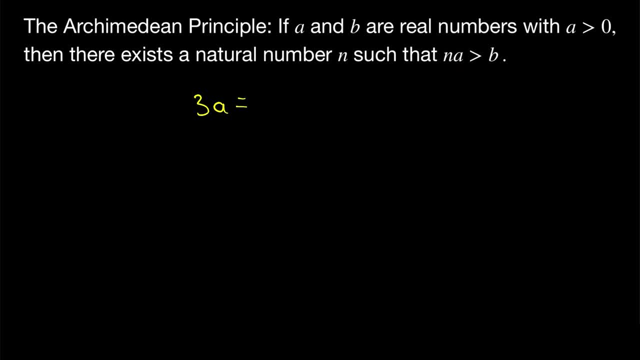 basically just adding A to itself N times, For example, 3 times A, is equal to A plus A plus A. So another way to think of this result is that if we have two real numbers, A and B, and A is positive, then we can add A to. 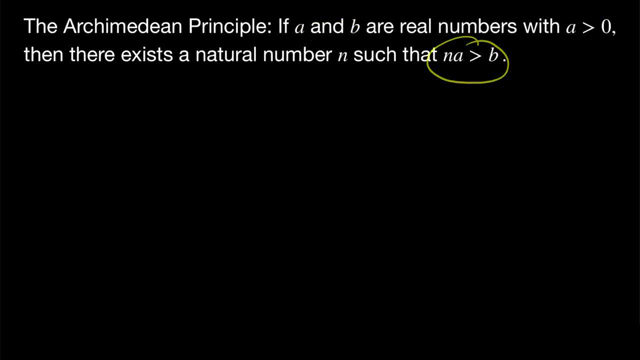 itself enough times to eventually surpass B. I think you'll agree that this is such an obvious fact that it's pretty cool. we can actually prove it. So let's see how the proof goes Quickly. we're going to reformulate what we're trying to prove, which will make the proof easier. 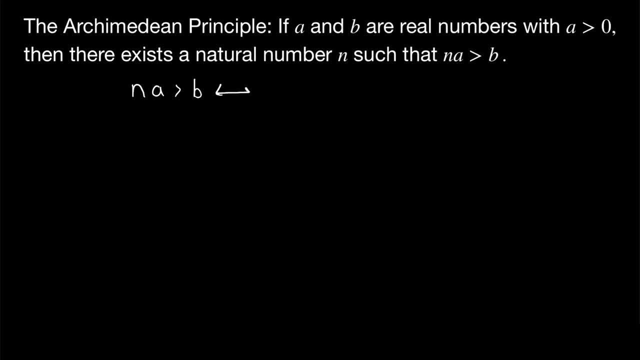 Certainly, if N times A is greater than B, well, that's the same as saying that N is greater than B divided by A, just dividing both sides of this inequality by A, which we know we can do with no complications Because A is positive. Now, what is B over A? Well, B over A is just a real number, Take care to note. 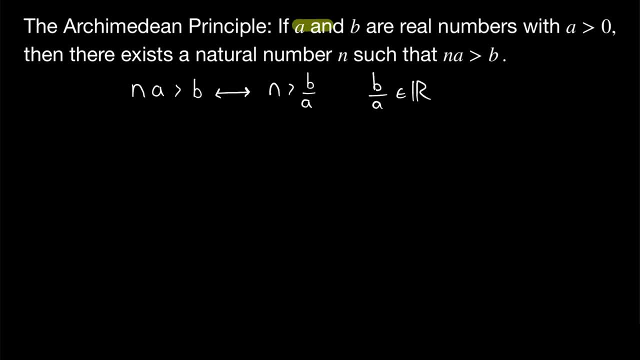 that it's not necessarily a rational number, because A and B are not necessarily rational numbers. They're just real numbers, So their quotient is also a real number, Since, again, we know that A isn't zero. Note that we could write any real number in this way, Just for. 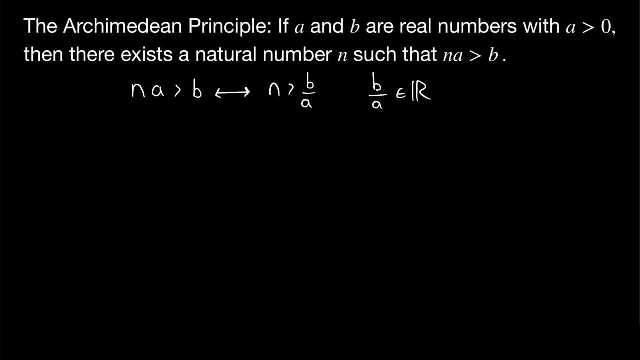 example, consider a real number: X. set B equal to X, A equal to Y and B equal to Y, So we can have X written in this form. In other words, we can simplify the problem. to this We want to prove. 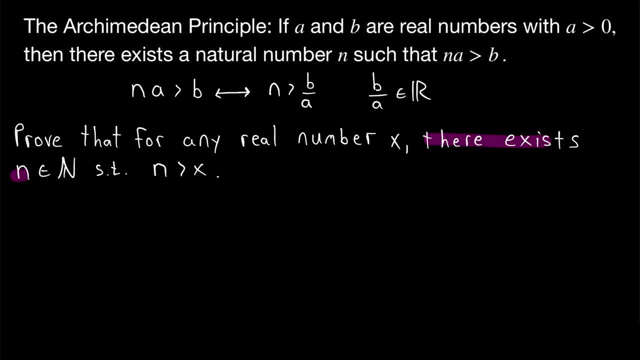 that for any real number X, there exists some natural number greater than X. This means that the natural numbers are not bounded above by any real number. Once more, just to emphasize how proving this is the same as proving the original form, given real numbers A and B with A greater. 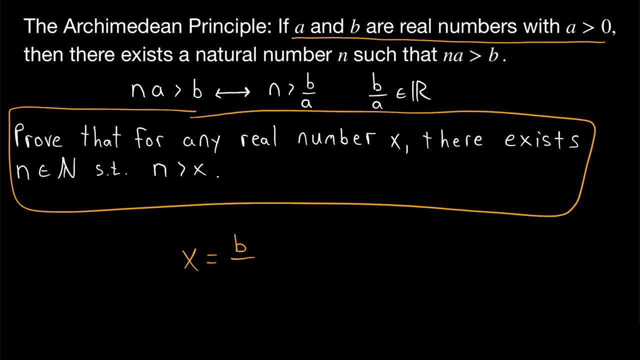 than zero, I can just set X equal to B over A, which is the same as proving the original form. So by this result that we're about to prove, we know there exists a natural number, N, greater than X, which is equal to B over A. So N is greater than B over A, And thus, of course, N times A. 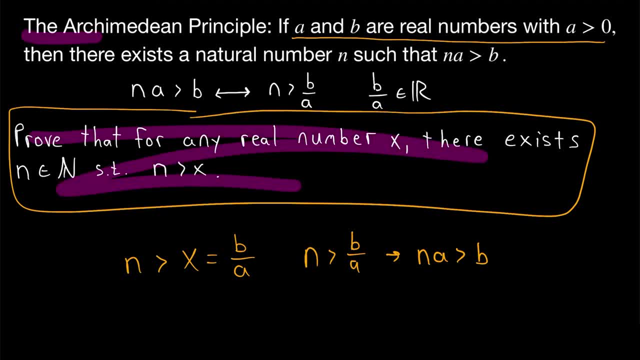 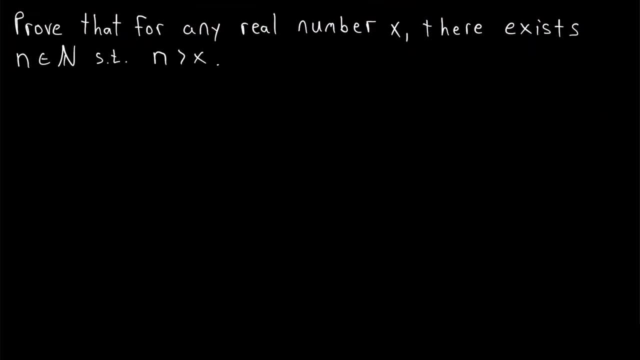 is greater than B. So by proving this we guarantee the original result as well. All right, no more dilly-dallying, Let's get right into the proof And we'll proceed by contradiction. We want to prove that for every real number X, there exists some greater natural number. So 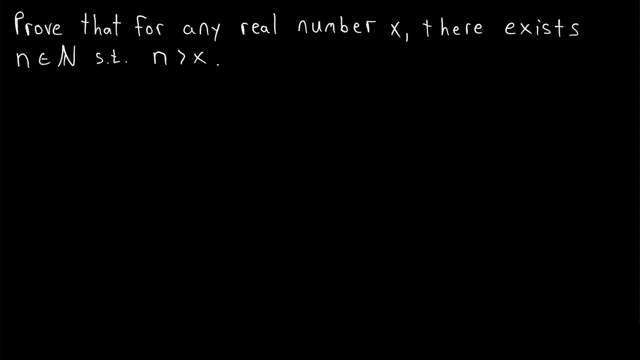 we'll assume for contradiction that there's some real number for which this doesn't hold, a real number that's greater than or equal to every natural number. So we say: suppose for contradiction, SFC, that there exists some real number X, such that X is greater than or equal to. 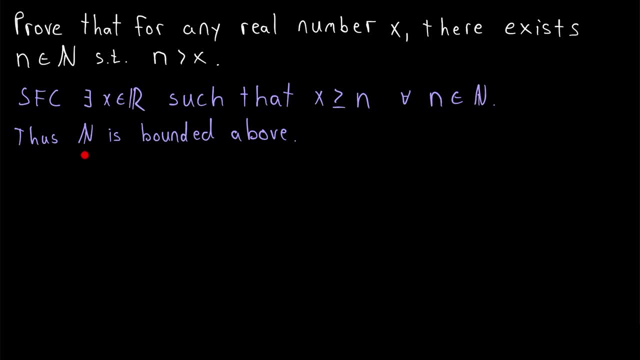 N for every natural number, N. Thus the set of natural numbers is bounded above. Also, we of course know that the set of natural numbers is non-empty. Thus, by the completeness of the reals, often called the least natural number, we know that the set of natural numbers is non-empty. 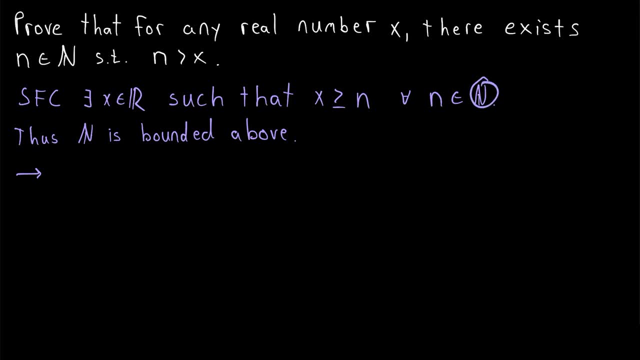 upper bound property. Since the natural numbers is a non-empty subset of the real numbers, that's bounded above, we can conclude that it has a supremum. The supremum of the natural numbers exists. Let's say it's equal to S. Then if the supremum of the natural numbers is equal to S, 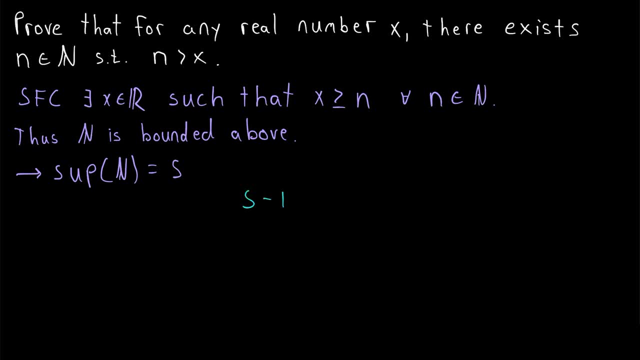 what do we know about, say S minus 1?? Well, certainly, by definition of supremum, S is the least upper bound of the natural. So if the supremum of the natural numbers is equal to S, so if we reduce it by subtracting 1, this S minus 1 is not an upper bound of the naturals. 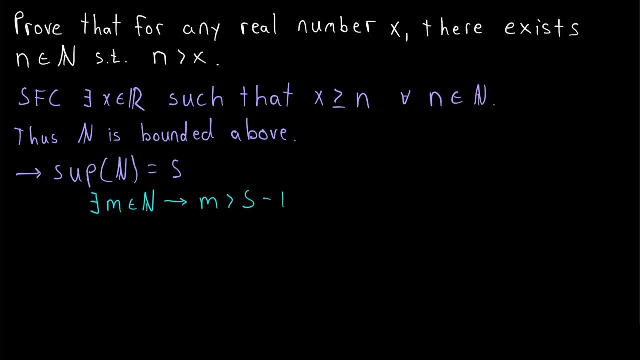 Hence, there must exist some natural number, say M, that is greater than S minus 1.. Since M is greater than S minus 1, we can add 1 to both sides of the inequality to conclude that M plus 1 is greater than S. And this, my friends, is a contradiction. It's a contradiction because M is a natural number. 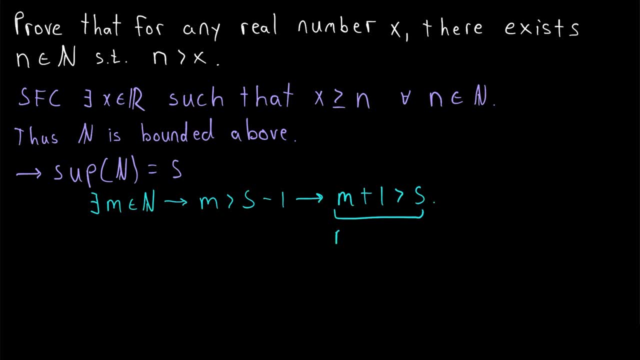 M plus 1 is also a natural number and the natural numbers are closed under addition. So M plus 1 is also a natural number, But that means we've found a natural number greater than the supremum of the natural numbers, which contradicts the definition of the supremum being an upper bound Hence, 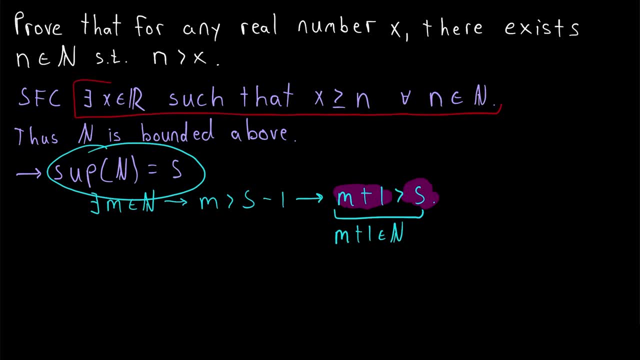 our assumption that there exists some real number that's greater than or equal to every natural number must be false, And thus, since there cannot exist a natural number greater than or equal to every natural number, we know that for any real number, there must exist a greater natural number.